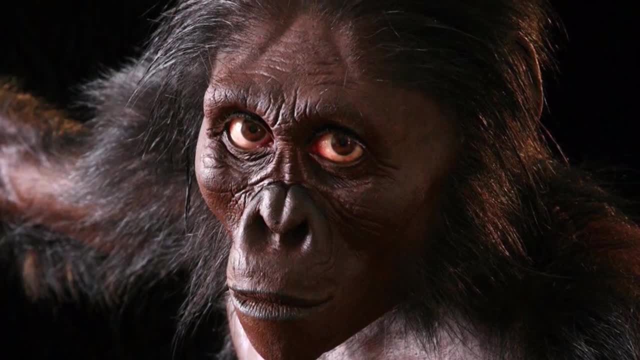 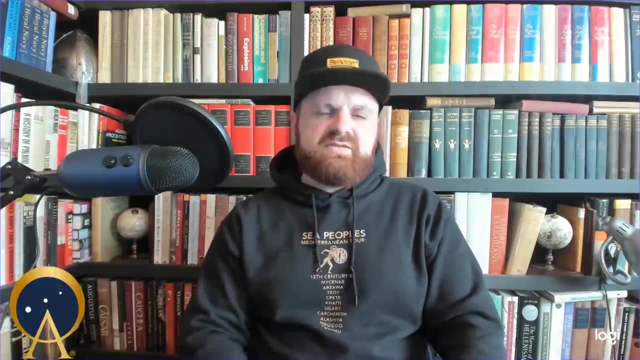 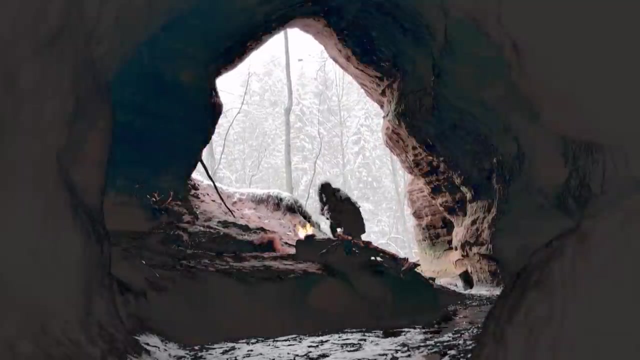 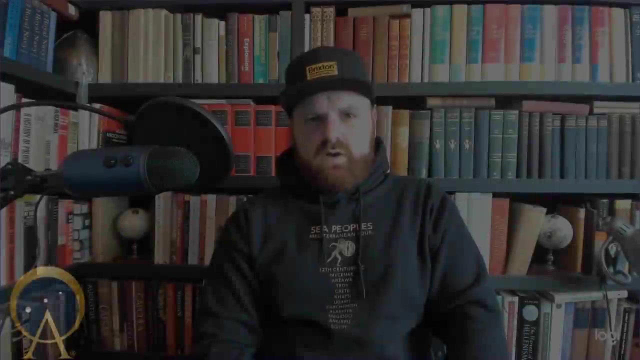 El Greco from Mediterranean Europe, Suggests that mankind emerged in Europe and not in Africa. This new study could completely rewrite and reshape human history and possibly forever leave behind the out-of-Africa theory. And so is the out-of-Africa theory in serious doubt. 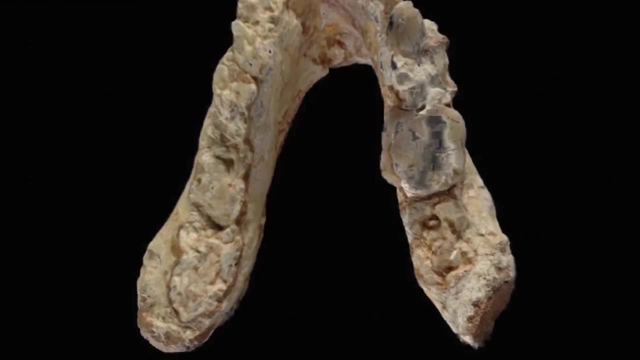 When an ancient toothy lower jaw was discovered back in 1912, it was discovered that the lower jaw of an ancient toothy lower jaw was a fossil. In 1944, in Greece, nobody really paid attention to the fossil as the casualties in Greece. 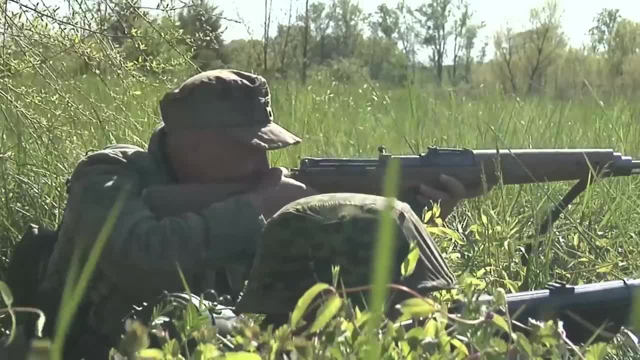 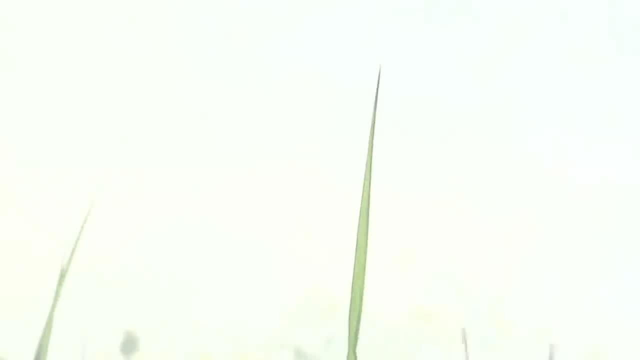 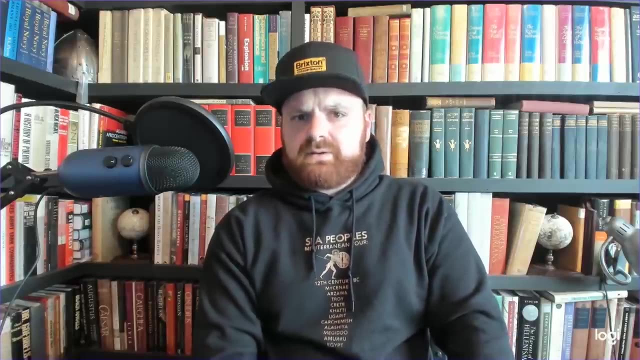 from the Second World War were so catastrophic that the extremely significant discovery was literally ignored by most anthropologists. When it comes to modern human origins, the out-of-Africa hypothesis has remained the dominant theory for decades. The theory suggests that every living human being is 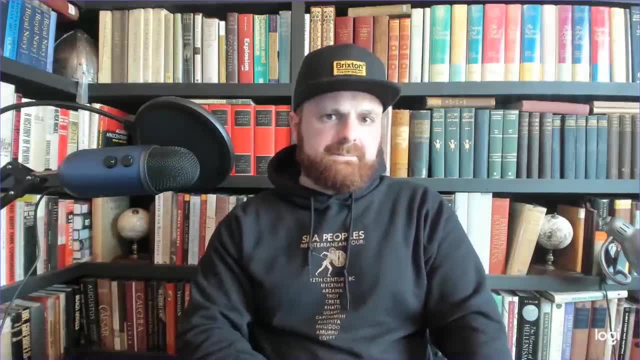 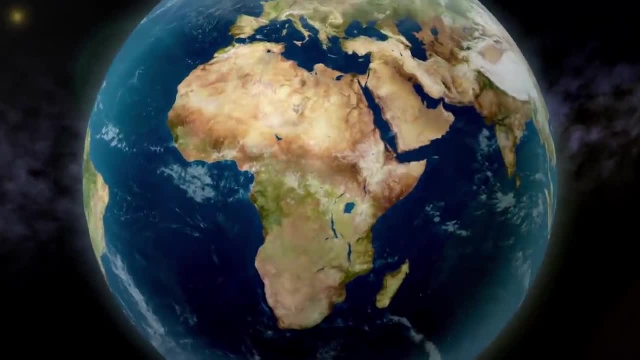 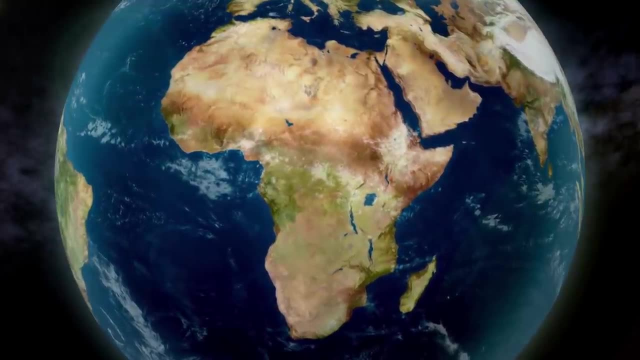 descended from a small group in Africa who then dispersed into the wider world, displacing earlier forms such as Neanderthals and Denisovans. However, according to Sky News reports, the birthplace of modern human beings may have been in the eastern Mediterranean rather than Africa. 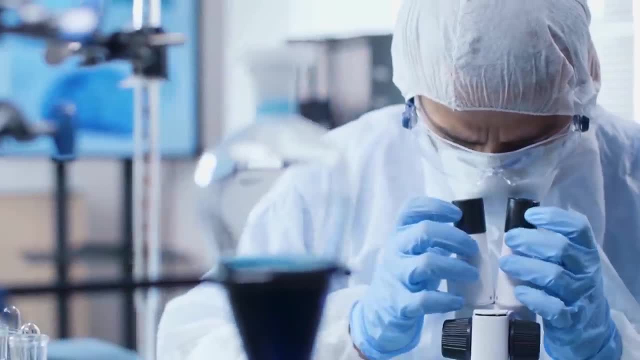 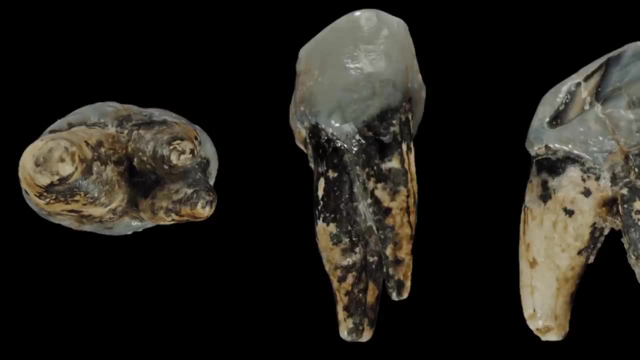 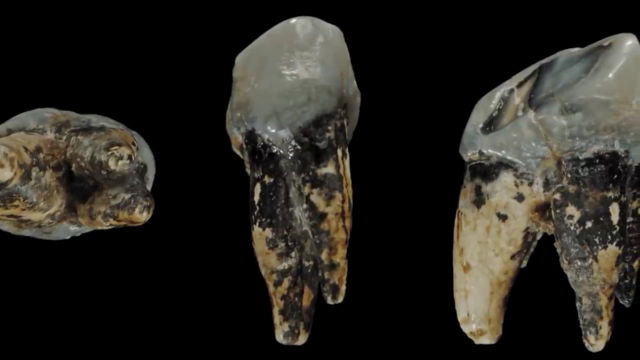 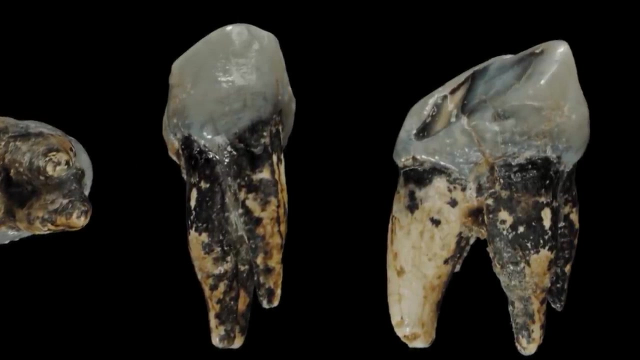 As an international team of scientists studying the ancient fossils of a tooth and lower jaw bone now suggest. in 2012, the ancient jaw bone was joined by a fossilized premolar tooth uncovered in Asmakha, Bulgaria. Scientists suggest that the remains belong to an ape-like creature known as Graecopithecus. 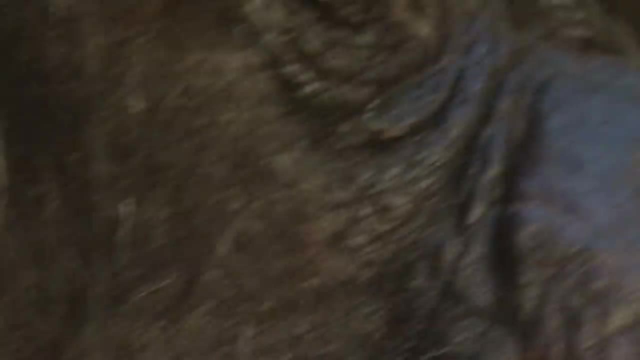 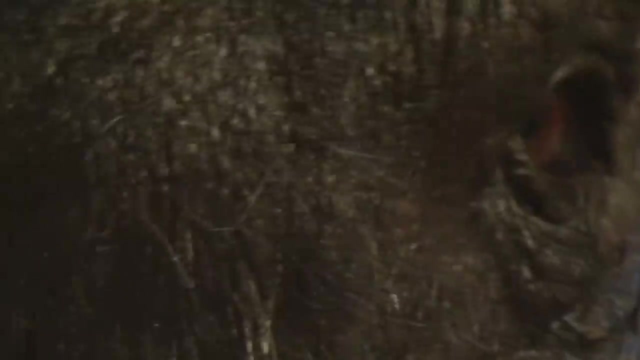 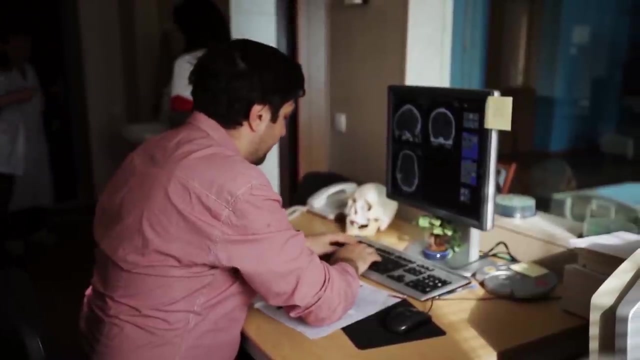 freybergii, which is now believed to be the oldest known pre-human, dating back as far as 7.2 million years. With the help of micro-computed tomography and 3D reconstructions of the roots and internal structure of the fossilized teeth, the researchers discovered distinctive features of contemporary 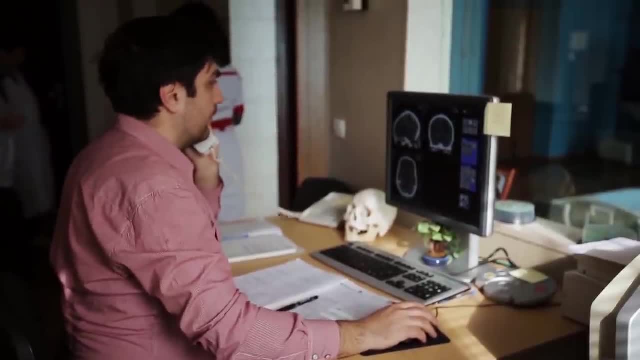 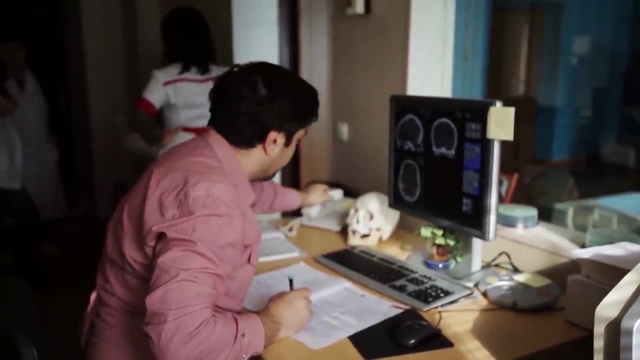 humans and their early ancestors. Project director Dr Bohm and Dr Spasov, along with their colleagues, examined both the Pyrgos fossil and the related upper pre-human teeth. The researchers discovered that the teeth of the Pyrgos fossil. along with their colleagues, 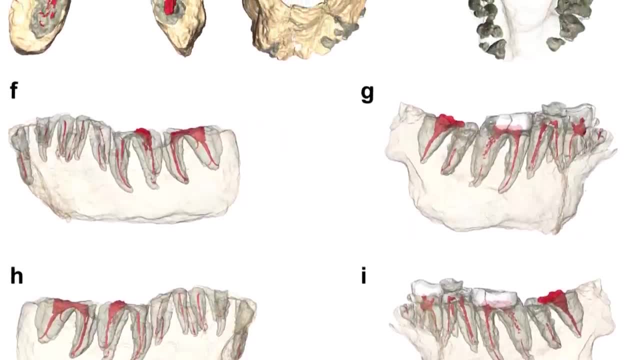 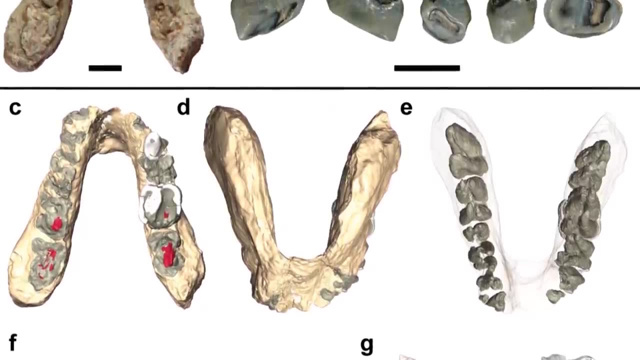 examined both the Pyrgos fossil and the related upper pre-human dating back as far as 7.2 million years, They came to the conclusion that El Graeco is the oldest known potential hominin. Dr Spasov stated that the fossil this hominin is several hundred thousand years older than. 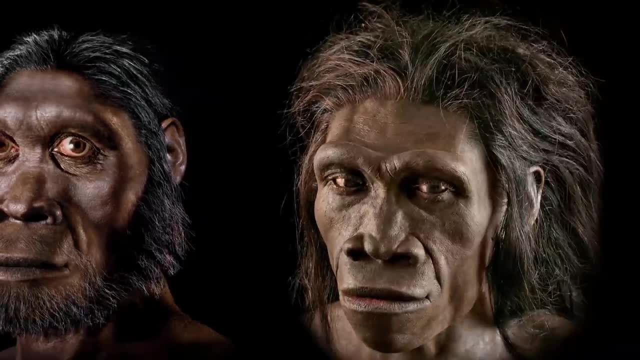 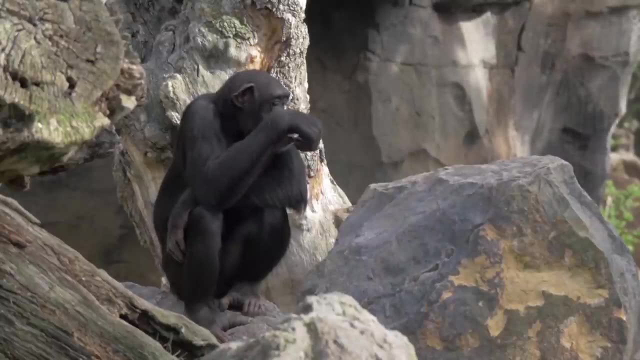 the oldest potential pre-human from Africa. Anthropologists refer to El Graeco as hominin or pre-human, for now, because the last common ancestor of modern humans and chimps retained both non-human pre-human and pre-human, pre-human, primate and human characteristics. 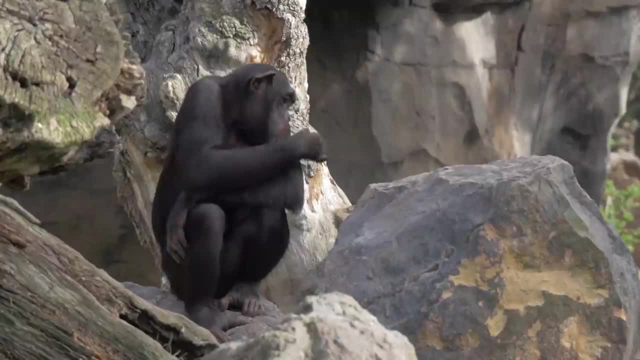 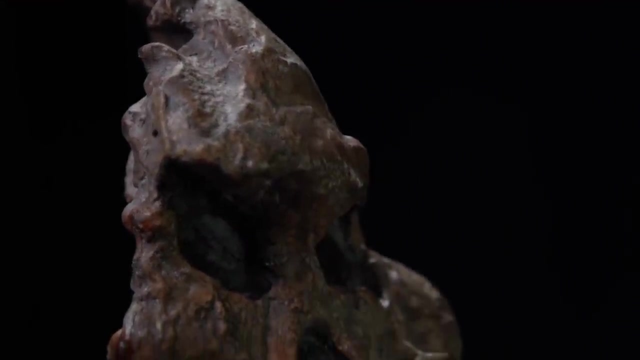 However, with the help of computer tomography, Bohm and her colleagues noticed that El Graeco's features were evolving into more modern-like human forms. Dr Bohm stated, while great apes typically have two or three separate and diverging roots, 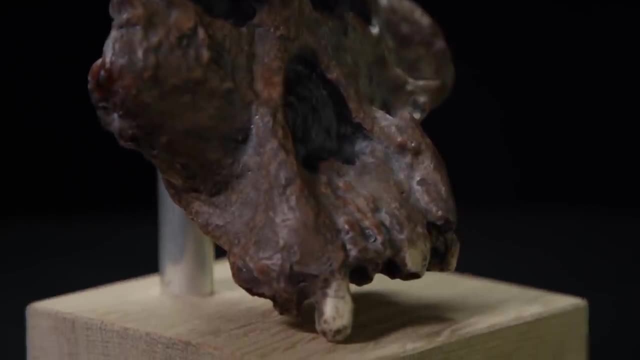 the roots of Graeco pythicus converge and are partially fused, Dr Bohm said, while great apes typically have two or three separate and diverging roots. the roots of Graeco pythicus converge and are partially fused, Dr Bohm said, while great apes typically have two or three separate and diverging roots. 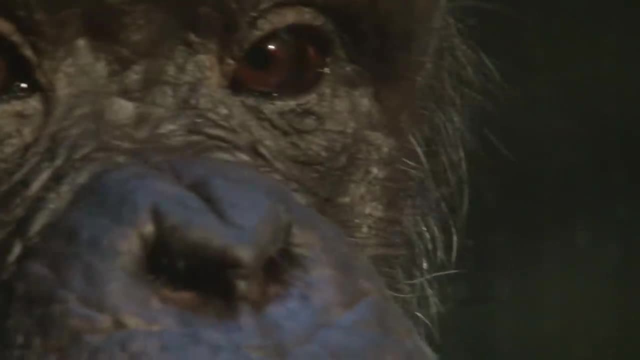 the roots of Graeco pythicus converge and are partially fused, Dr Bohm said. while great apes typically have two or three separate and diverging roots, the roots of Graeco pythicus converge and are partially fused, A feature that is characteristic of modern humans, early humans and several pre-humans. 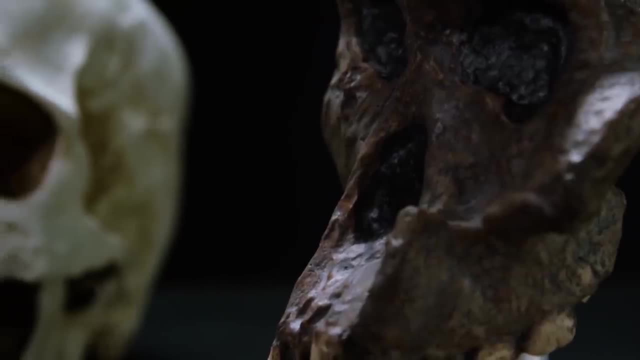 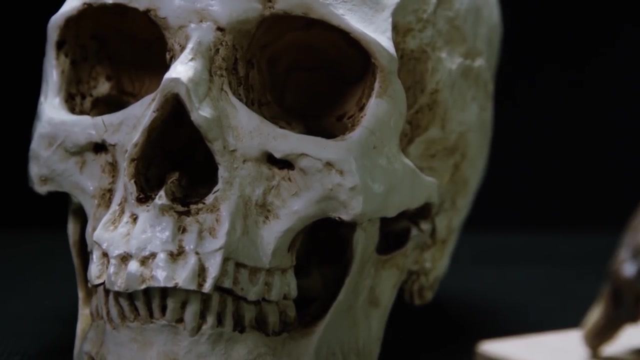 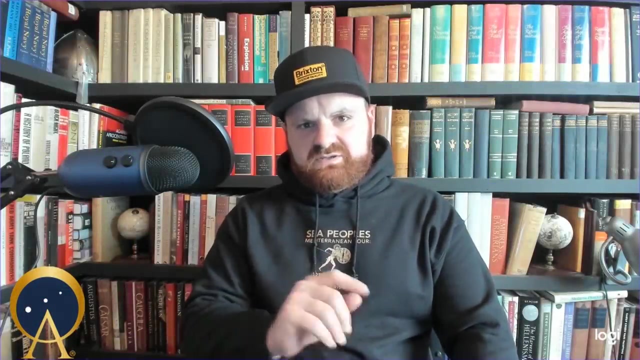 including Ardipithecus and and Australopithecus. Furthermore, one of the researchers, Dr Begone from the University of Toronto, believes that if we move Graeco pythicus to our own line, then mankind's history could be rewritten. 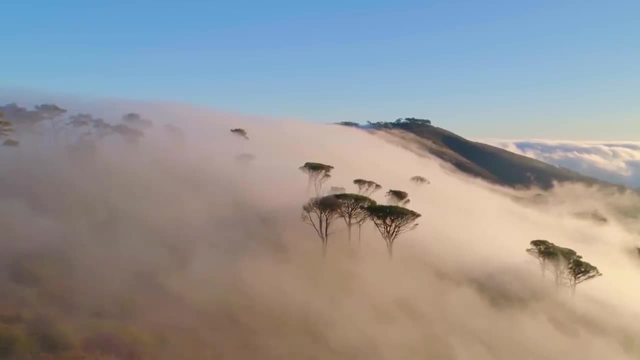 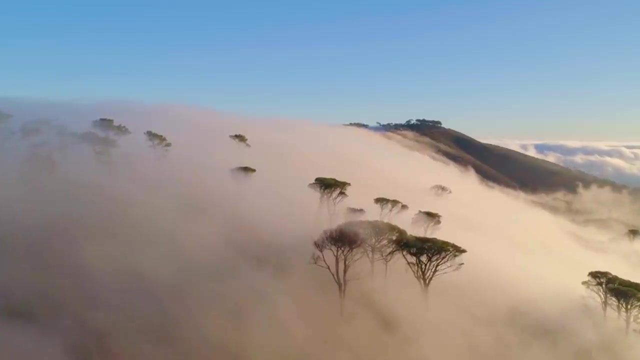 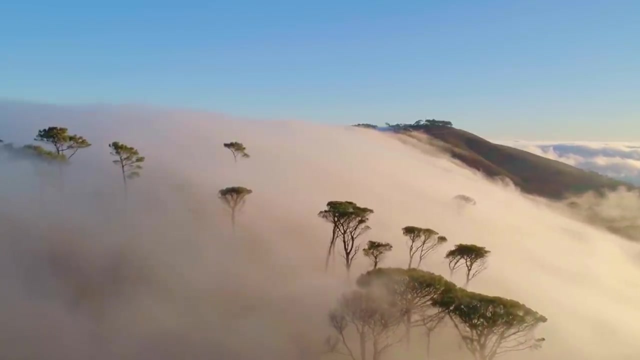 He told Science Alert. If this is indeed a human, it would be the oldest human ancestor known and the first to be identified outside of Africa Ever since Darwin. conventional wisdom is that the last common ancestor of chimpanzees and humans lived in Africa. 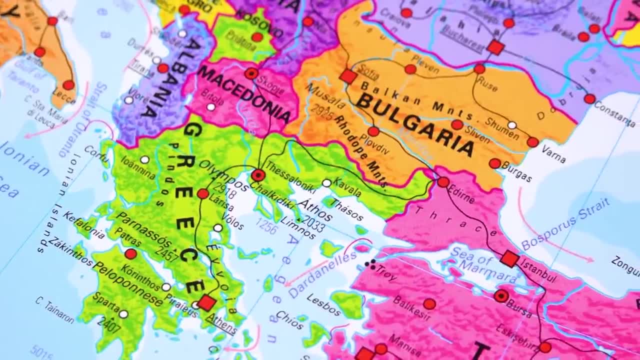 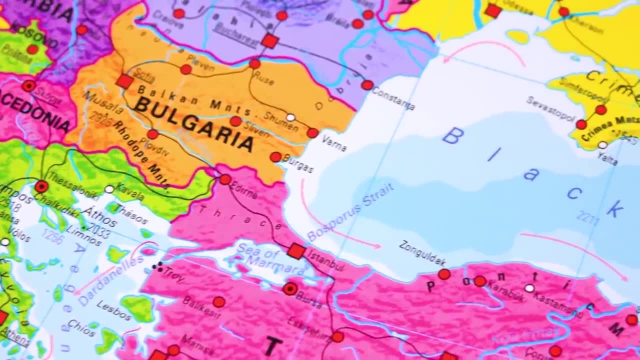 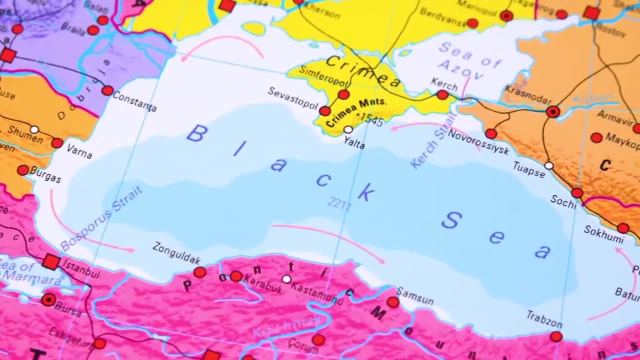 He went on to state that our research shows that the earliest humans may have actually evolved in Europe. Although Dr Bohm appears to be confident that El Greco's ancestors are Eurasian hominins, such as Ouranopithecus from Greece, she and her team are not ruling out the scenario that 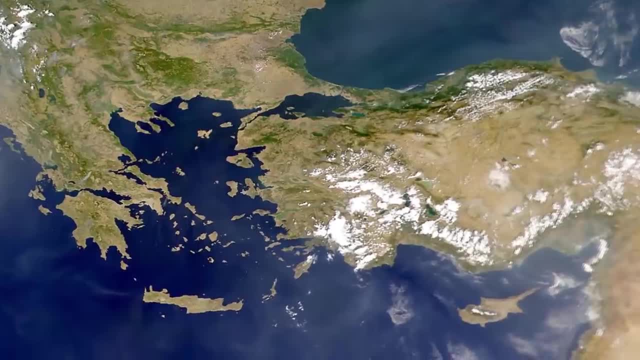 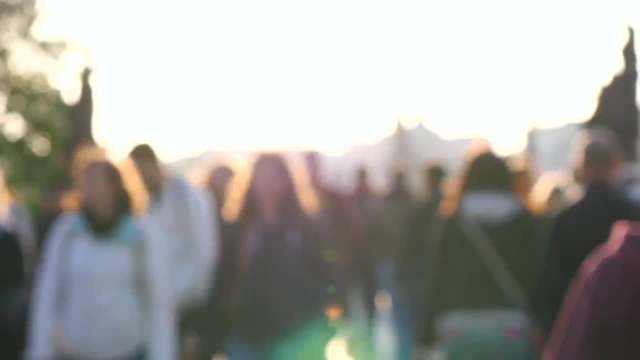 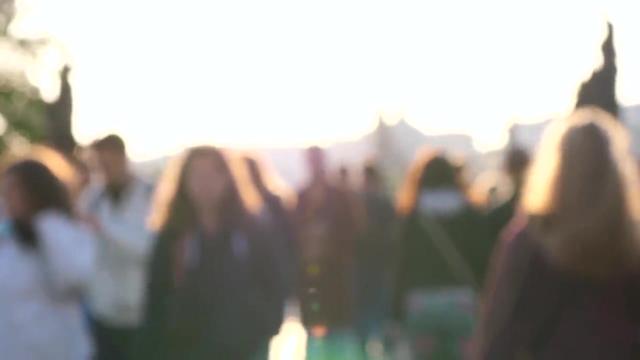 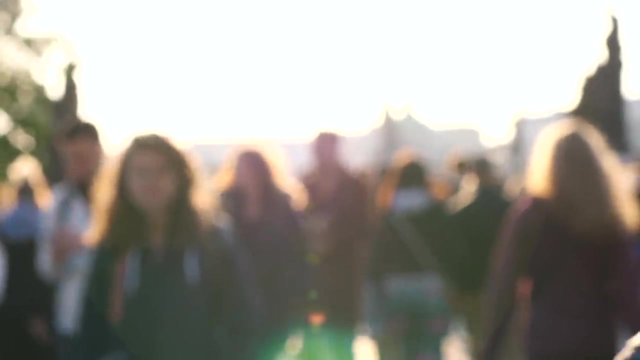 some of his descendants possibly migrated to Africa at some point. Of course, they consider it most possible that several of his descendants, as well as other early pre-humans, remained in the Mediterranean and spread throughout Europe and Asia. If this theory is true, then it's very possible that his descendants could have evolved into: 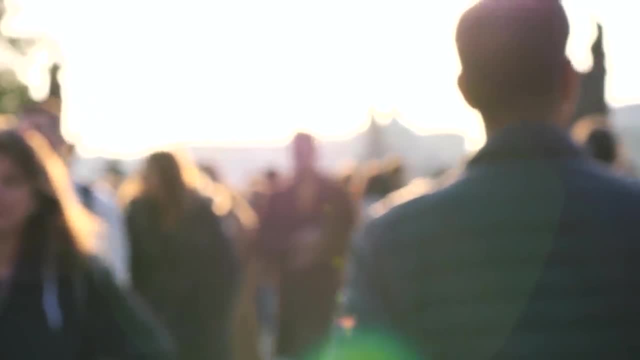 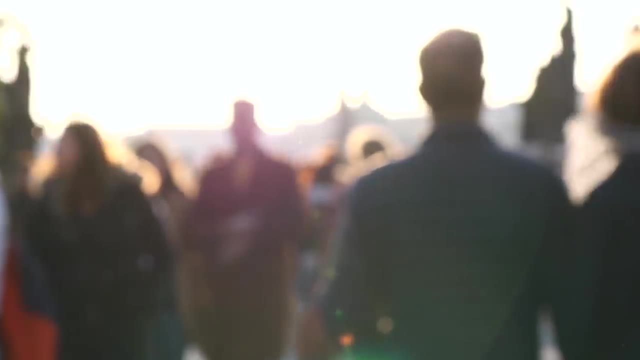 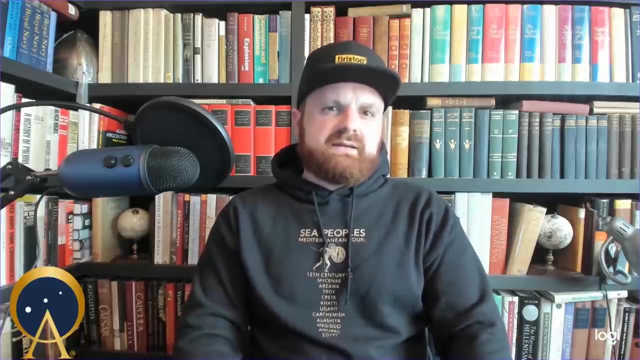 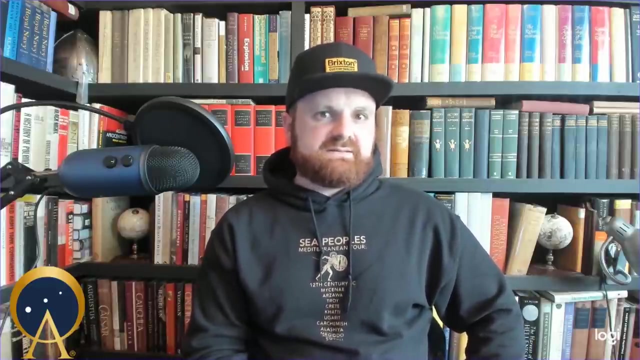 Neanderthals, Denisovans and the other early humans known from these geographical areas that are directly related to people of European and Asian origins. Today, the only sure thing is that if more evidence confirms such theories, in the future human history as we know it would drastically change. 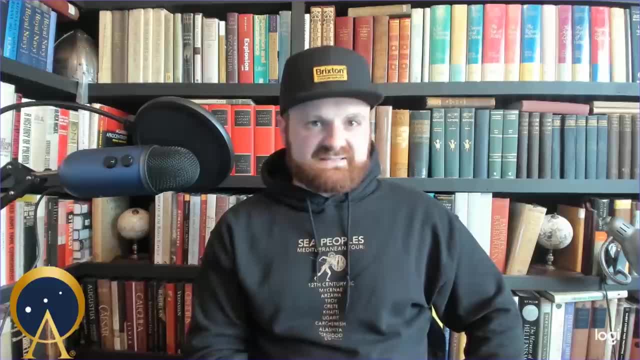 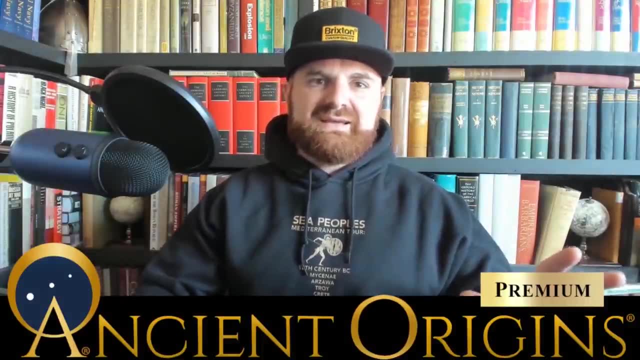 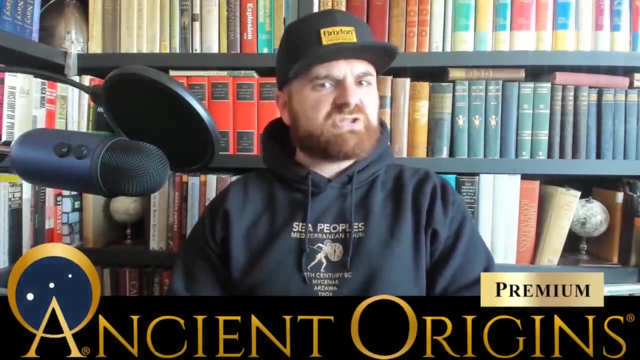 As Dr Spasov said, our new hypothesis is a smoking gun. Ladies and gentlemen, welcome to the Study of Antiquity and the Middle Ages. As always, I am your host, Nick Barksdale, and today I'm bringing you a very special 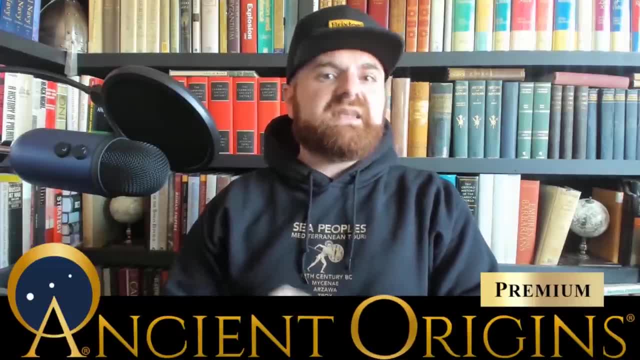 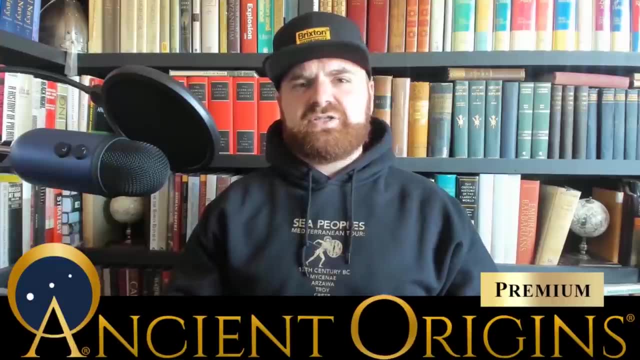 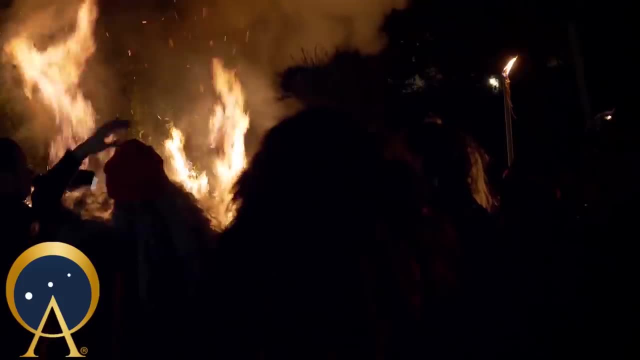 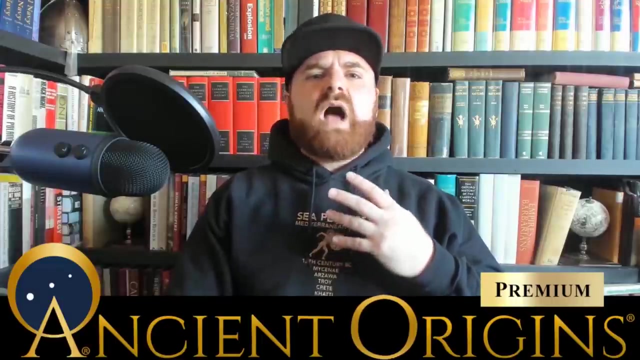 episode. This episode is brought to you by none other than Ancient Origins. Ancient Origins specializes in reconstructing the story of humanity's past And, honestly, for those of you who love anything ancient, mysterious and the unexplained, it's the best resource online for you, providing a variety of content. 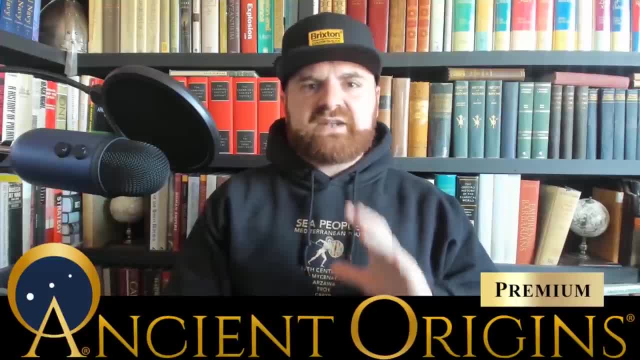 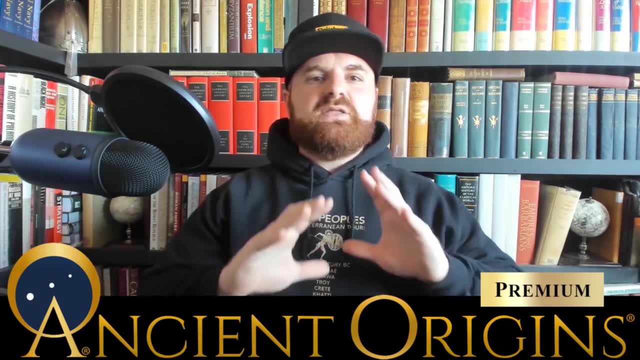 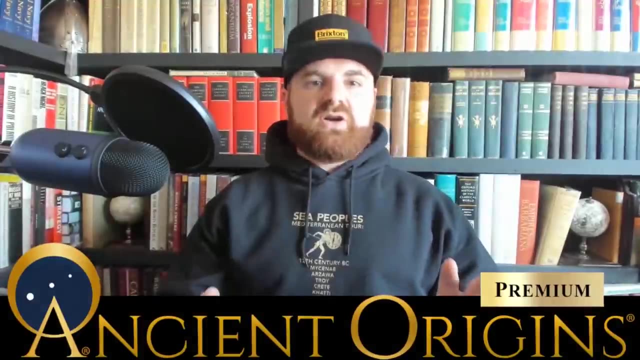 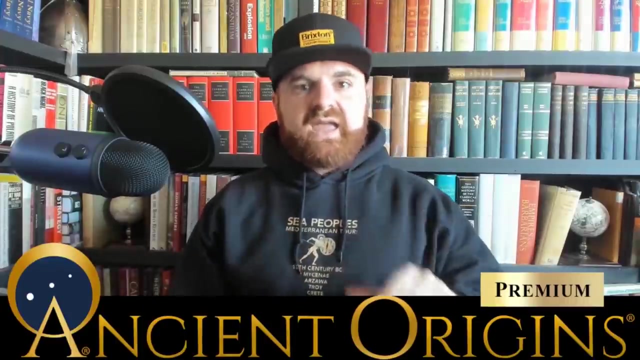 But more importantly, it's helping us understand the subjects that we all love, From the fringe to the mainstream. you get the best of everything, But if you want access to even greater content, I highly suggest you becoming a premium member. to Ancient Origins.